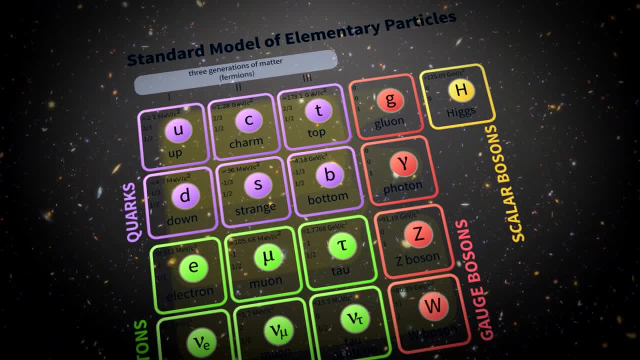 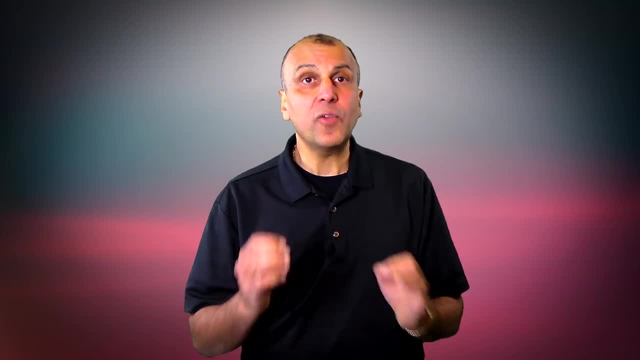 by the standard model of particle physics. It's a stunning piece of work which explains nearly everything, but it has a gaping flaw, because it does not explain something that is fundamental to our existence. Not only that, it also happens to predict that our universe should not exist. 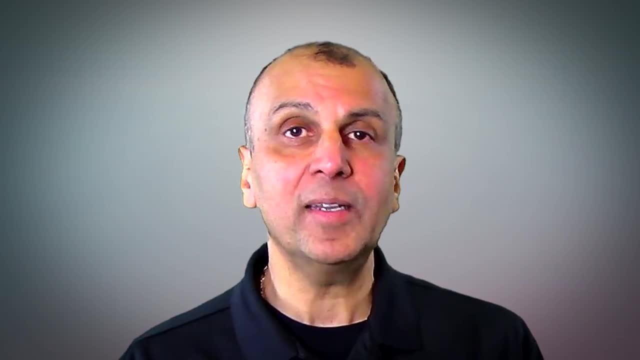 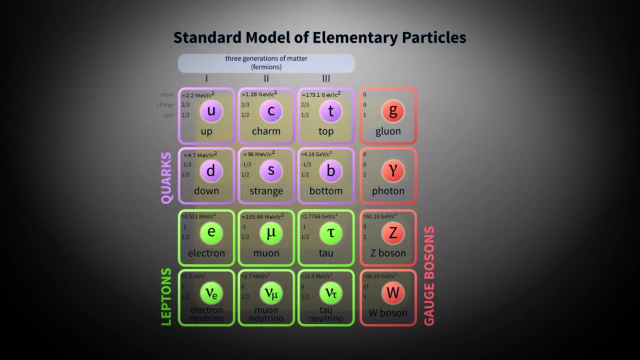 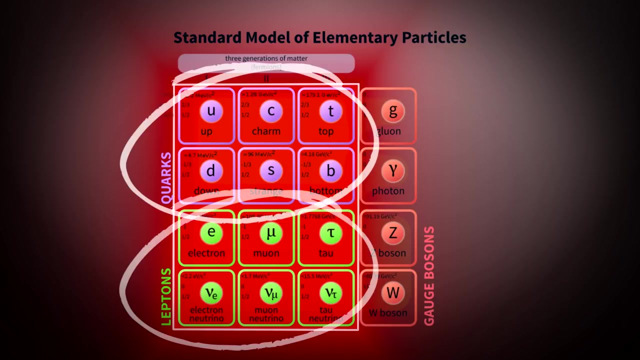 at all. What is the standard model and what does it not explain That's coming up right now. The standard model consists of twelve elementary particles known as fermions. The fermions are six quarks and six leptons. All non-fundamental particles are made of these. 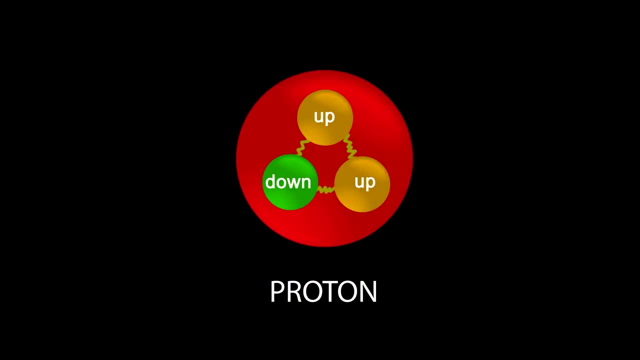 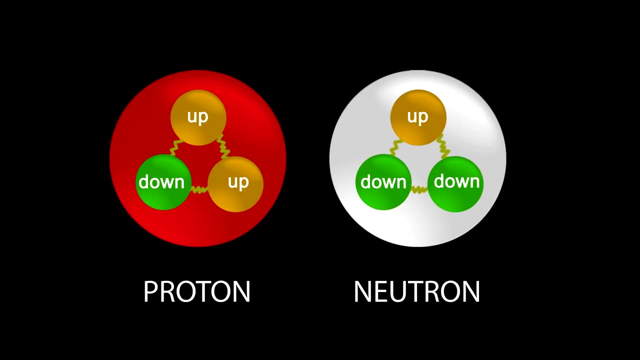 elementary particles. So, for example, A photon is made of two up and one down quarks, A neutron is made of one up quark and two down quarks. The gauge bosons are force carriers and are responsible for three fundamental forces of nature. 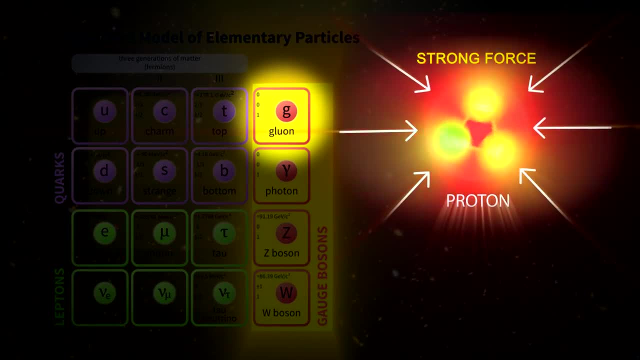 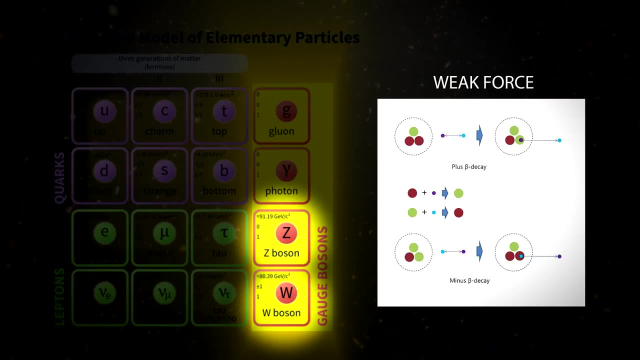 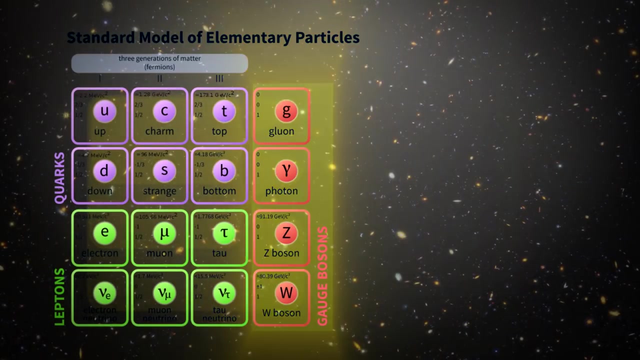 Gluons mediate the strong force which binds the nucleus of an atom. W and Z bosons mediate the weak force which is responsible for radioactive decay. Photons mediate the electromagnetic force which causes light and magnetism. The recently confirmed Higgs bosons give all fundamental particles their mass. 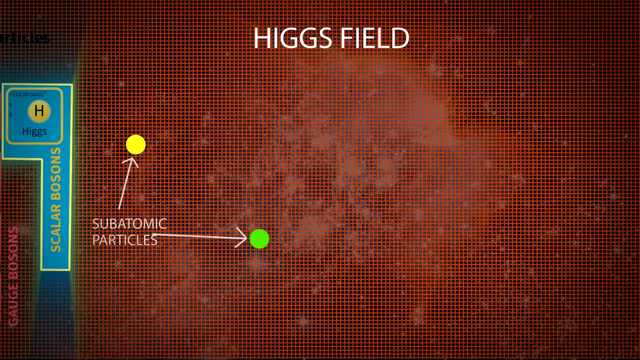 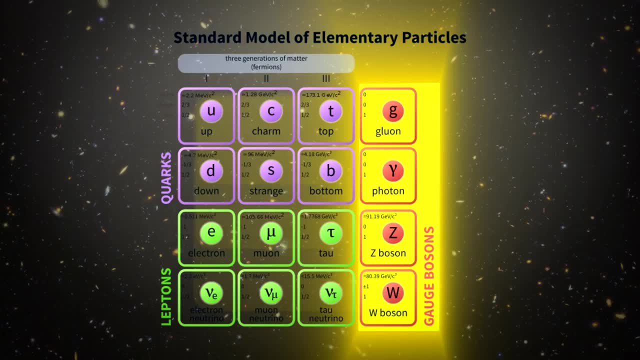 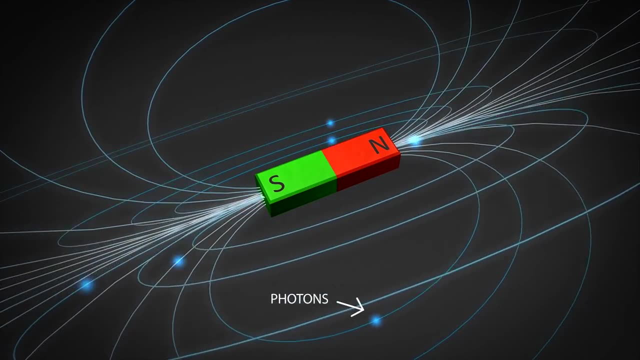 by interacting with them. Higgs does not interact with photons and gluons, Thus they are massless. G dod- Martha's theory, are ignorstalking us. I believe there is nothing harnessable we can do as a human being learned by nossas doughs. 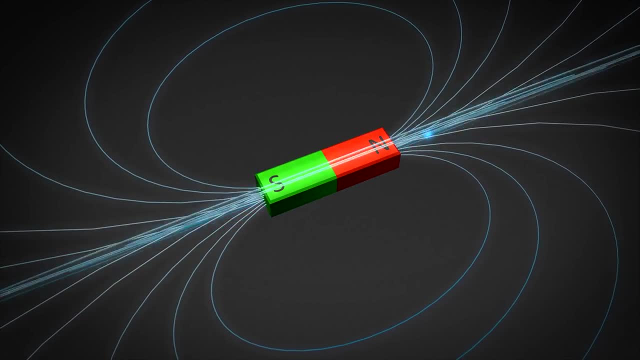 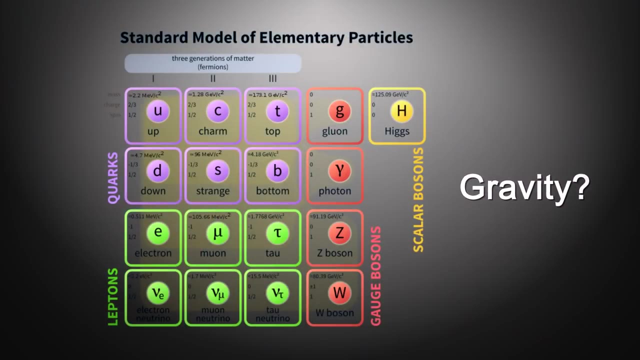 You can't see this with the naked eye, but they're there. Similarly, the other gauge bosons are being exchanged to manifest the other forces. Did you notice what's missing from the standard model? yet Where is gravity? It's nowhere to be found. 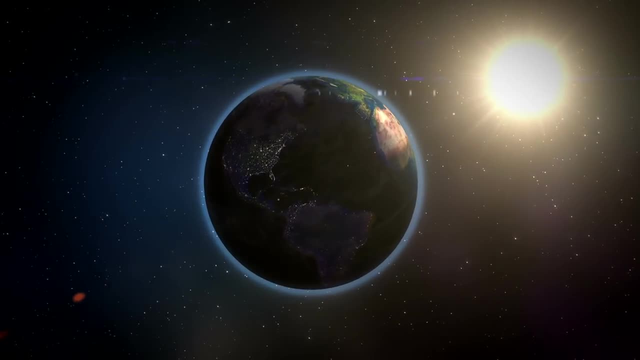 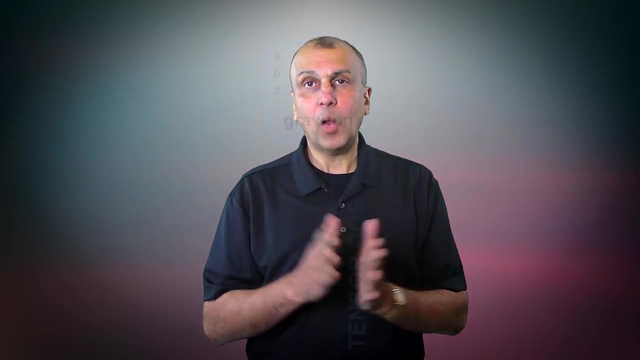 This is pretty important because, of course, without gravity the universe and we would not exist. So, as impressive as the standard model is, it does not explain gravity. You might say, well, all we have to do is find a new gauge particle called the graviton. 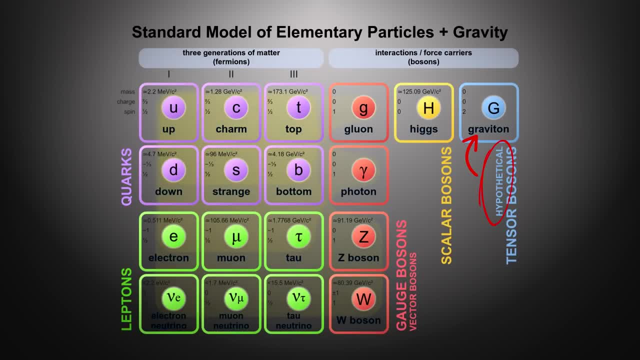 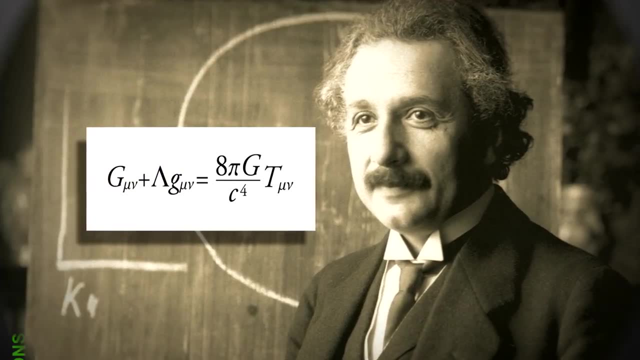 Then we'll have a model that explains everything right, Not so fast. Even if we found a theoretical particle called the graviton, it wouldn't completely explain gravitation. Our best explanation for gravitation right now is Einstein's general theory of relativity. 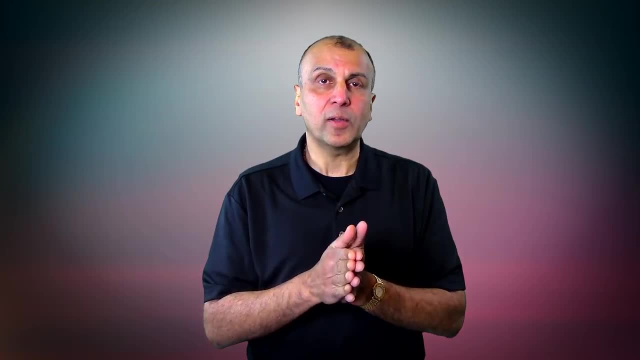 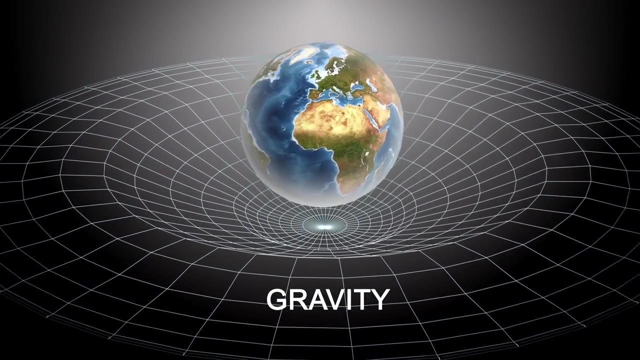 So why is gravity so difficult to integrate into the standard model? Well, unlike the other forces which can be explained using quantized particles, gravity does not necessarily even need a particle Because, at its fundamental level, it can be explained in geometric terms. You see, General relativity is about curvature of space rather than interaction of particles, At least that's what it appears to be. We can only presume that gravity must have a quantum form, But maybe it doesn't, We don't know. The other three forces don't seem to bend space and time. 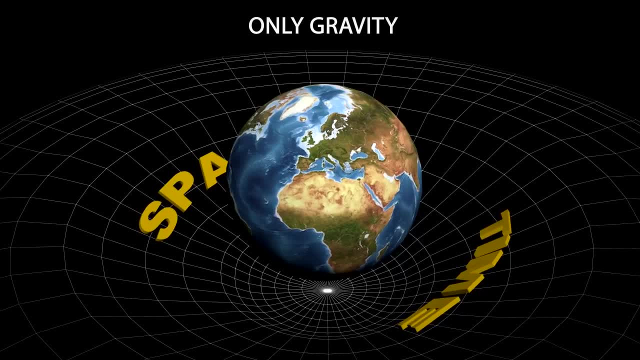 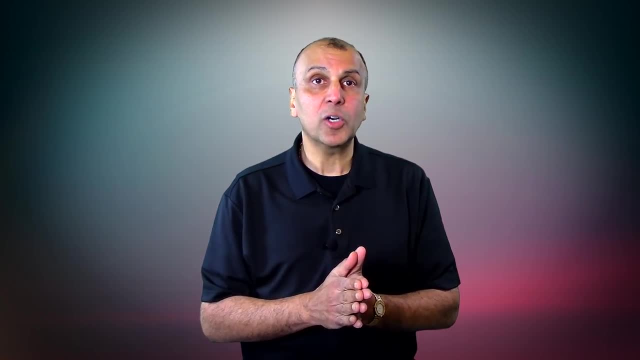 Only gravity does. So that is what so far, no one can explain and thus incorporate into the standard model. There are some leading theories that are attempting to put gravity in terms of the quantum world, Namely The theory of gravity and loop quantum gravity. 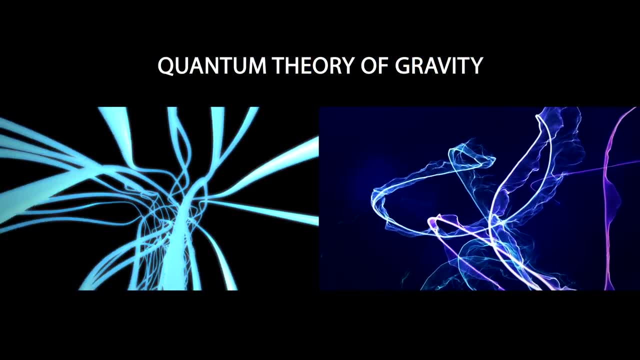 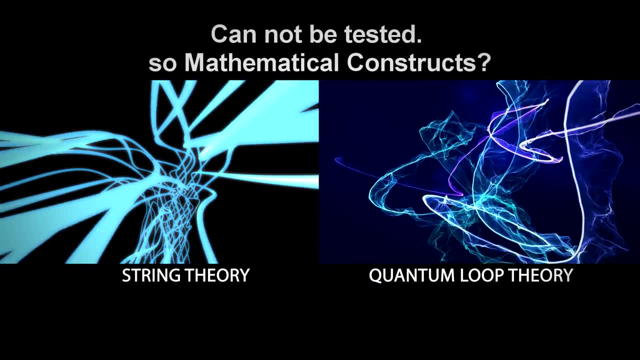 They provide the possibility of a quantum theory of gravity And according to these theories, a graviton must exist. But the major problem with these theories is that they don't make predictions that we can test. So for all intents and purposes, they may just be random mathematical constructs that 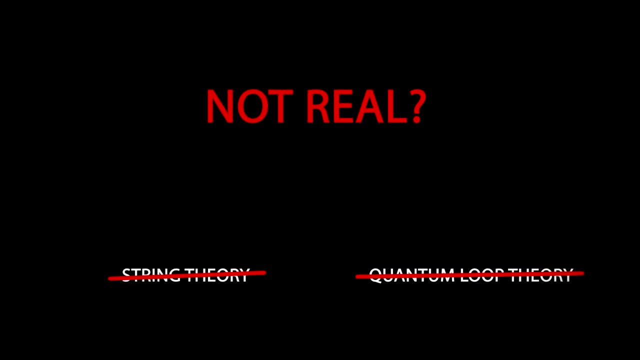 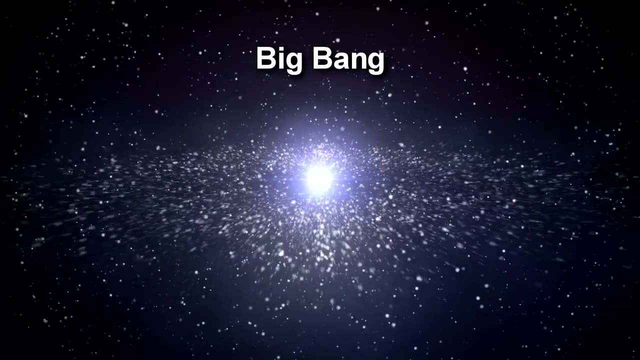 happen to model certain parts of nature. The theory of gravity breaks down at the quantum level, So we have no way to explain the singularity of a black hole or the events that led up to the big bang. But luckily, In particle physics, when it comes to the minuscule scale of particles, the effect of 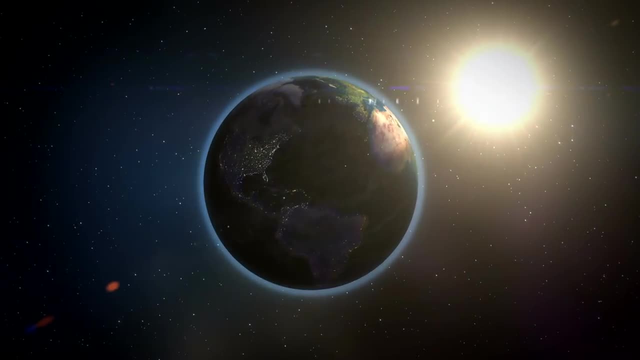 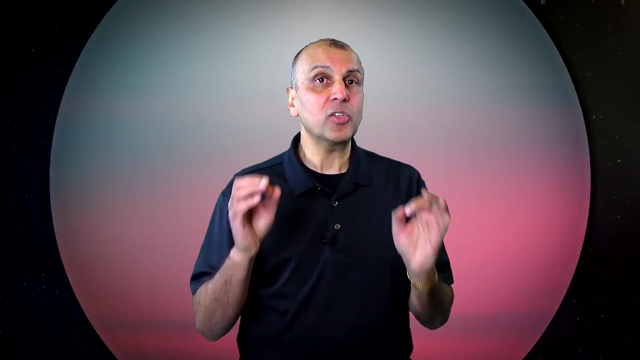 gravity is so weak that it is negligible. Only when matter is in bulk, at the scale of the human body or of stars and planets, does the effect of gravity dominate. So the standard model still works well, despite its non-explanation of a fundamental force. 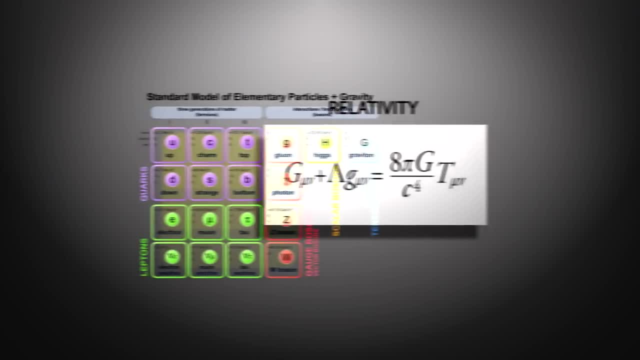 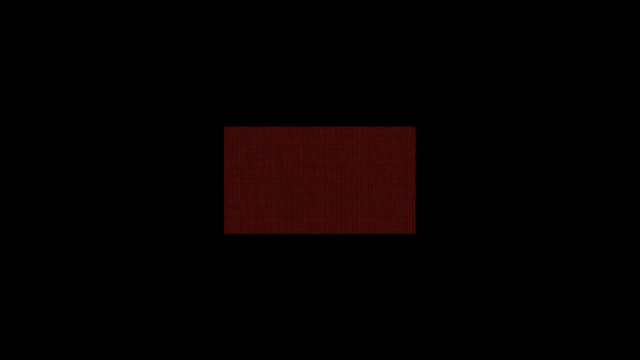 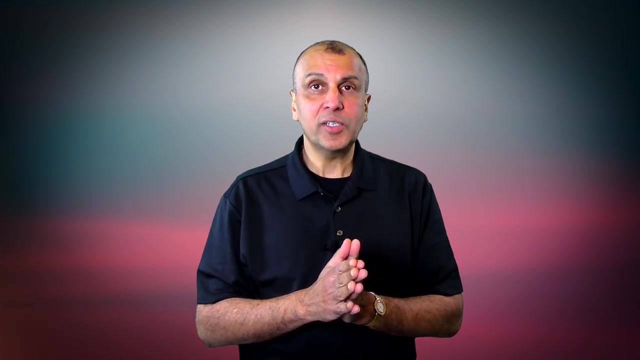 of nature. What we really need is a theory of everything that unites relativity and quantum mechanics. It's possible that space-time itself is not smooth, As general relativity presumes, But is itself made up of quantum particles. In any case, if the next Albert Einstein or Isaac Newton happens to be watching this video, 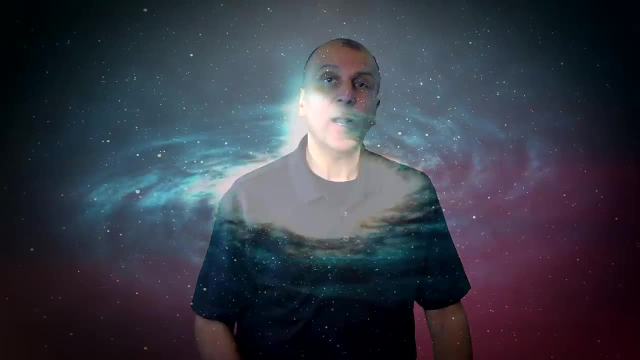 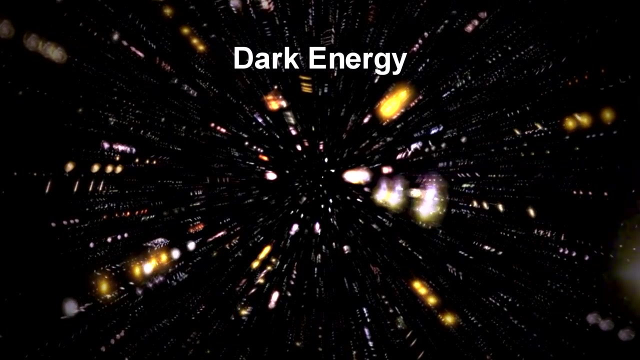 and is inspired to come up with a quantum explanation for gravity. perhaps he or she could also explain dark matter and dark energy, Because these are not explained by the standard model either. And lastly, according to this model, there is a certain problem of matter-antimatter. 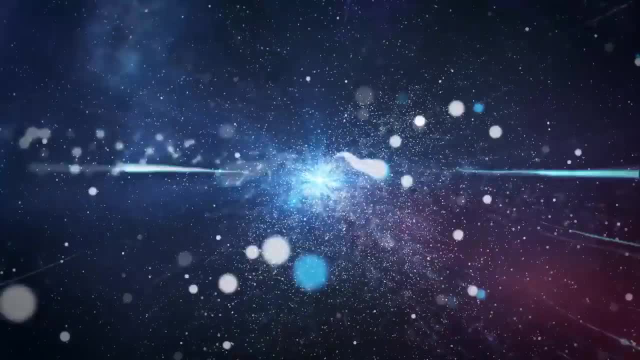 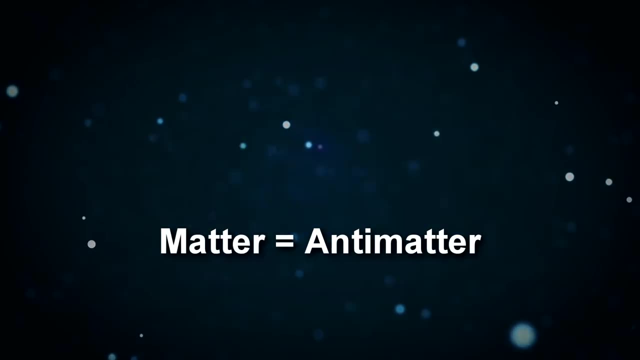 symmetry. You see, the model predicts that at the beginning of the universe, at the big bang, there should have been an equal amount of both things, Both matter and antimatter. That should have totally annihilated each other, so that the universe would be a massive.